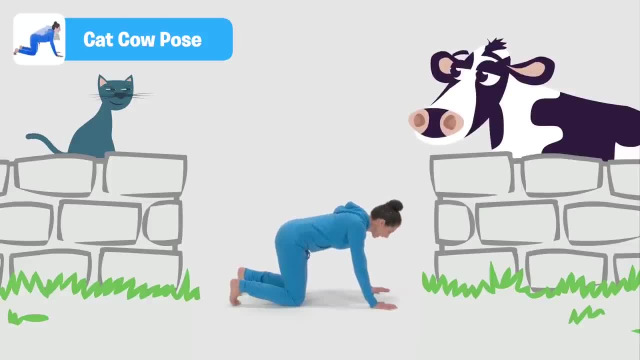 Let's try it again. Here we go: We're going to arch our back up, look into our tummy for our cat pose. Then we're going to dip our belly down, wiggle, waggle our tail and lift our chest for our cow pose. 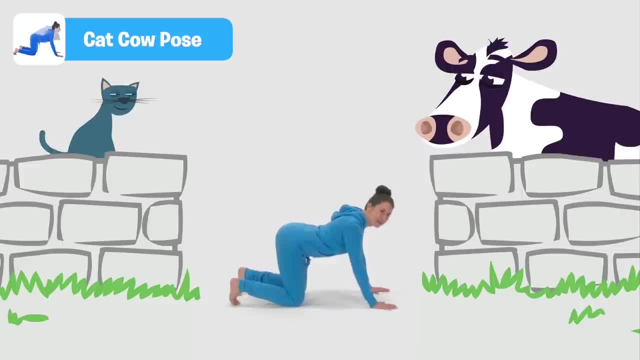 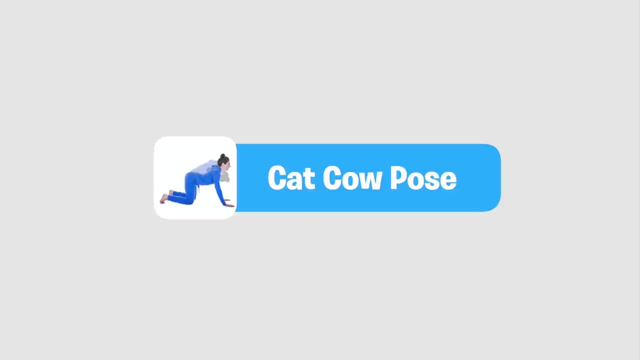 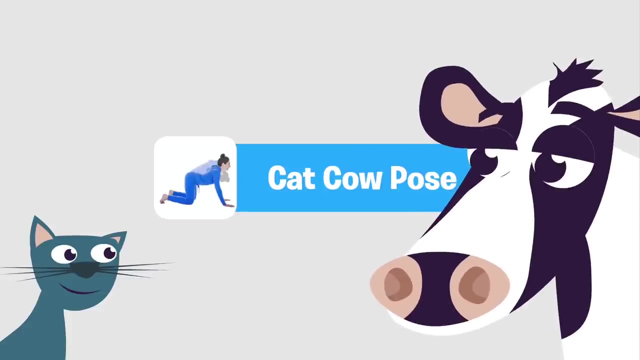 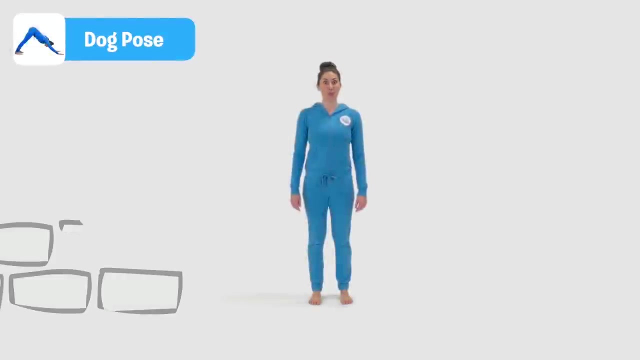 Now let's see if we can do four or five, Five in a row. Here we go. Cat Cow, Cat Cow, Cat Cow- Oh, I could do this all day long. Cat cow pose, Dog pose, Coming down onto our hands and our knees. 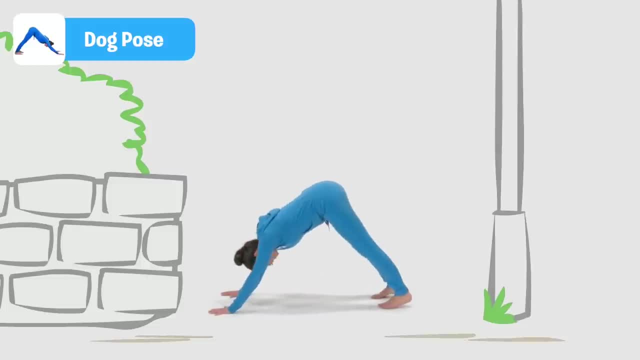 We spread our fingers wide, tuck our toes and press our hips up to the sky. Yes, Now look, there's a friend. Hello, Aww, that's nice Now. dogs always like to wag their tails when they're pleased to see you. 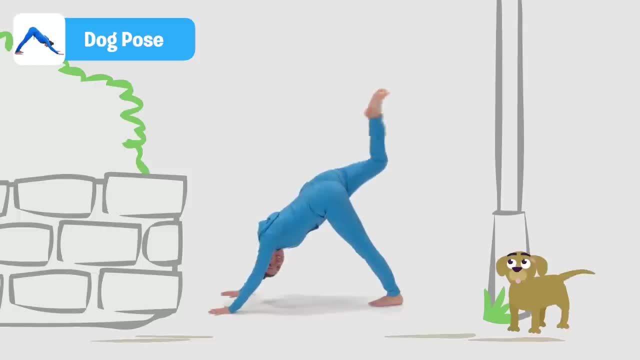 So let's try that. now We reach up with one of our legs and we give it a wag, Waggle, waggle, waggle. Very good, Lowering it back down Now. dog pose is very good for strengthening our arms and stretching the backs of our legs. 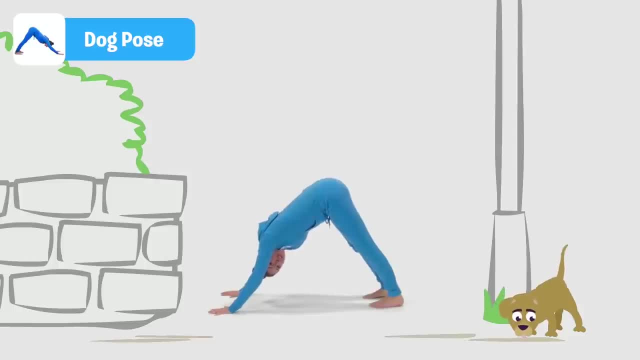 And because we're upside down, we get lots of lovely fresh oxygen to our minds, So it's very good when we're feeling a bit tired. Let's try wagging our tail on the other side now, Stretching our other leg up and giving it a wag. 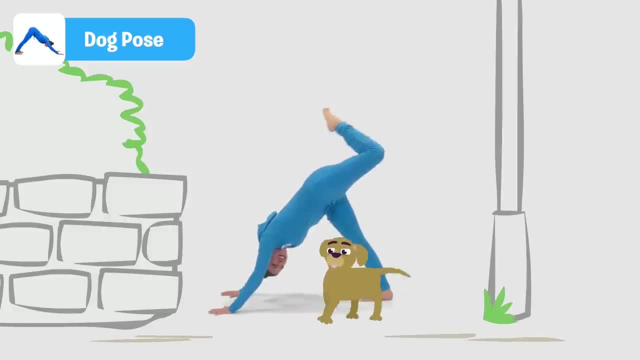 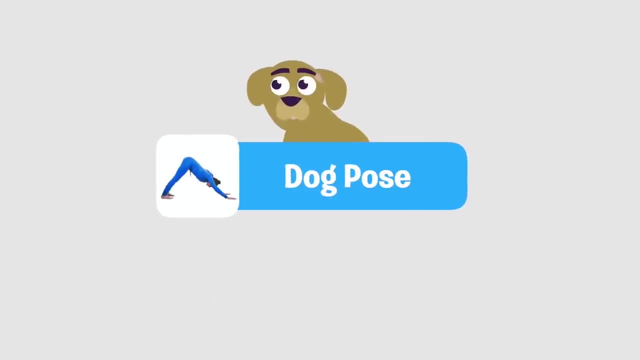 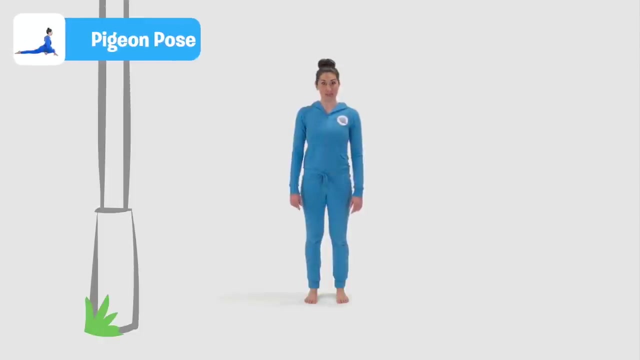 Waggle, waggle, wag. Oh, thank you, I love you too. Dog pose- Pigeon pose, Coming down to sit on our bottoms with our legs crossed. Now we take this front leg, stretch it forwards, sweep it all the way around the side to pop out long at the back. 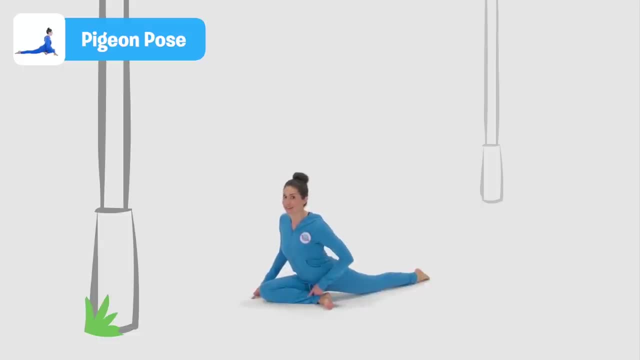 Keeping this front leg at a nice diagonal line. Now, using your fingers like tents, roll your shoulders back and puff up your chest like you're a proud pigeon Going coo, coo, coo. Better not do it too loudly or the pigeons will hear and maybe come and land on our heads. 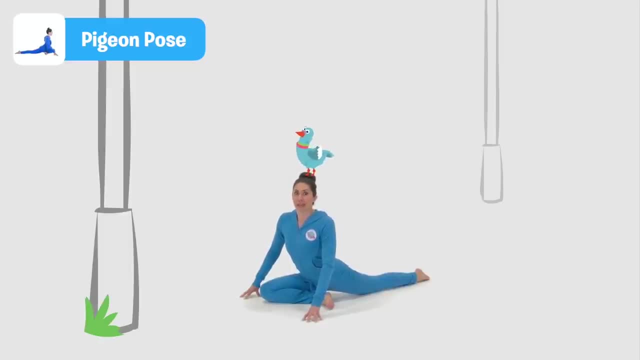 Oh good, Okay. so pigeon pose is really good for opening our hips and stretching our legs. It's also really good if you do a lot of cycling or running, Because it helps release those lovely tight muscles. Let's try it on the other side. 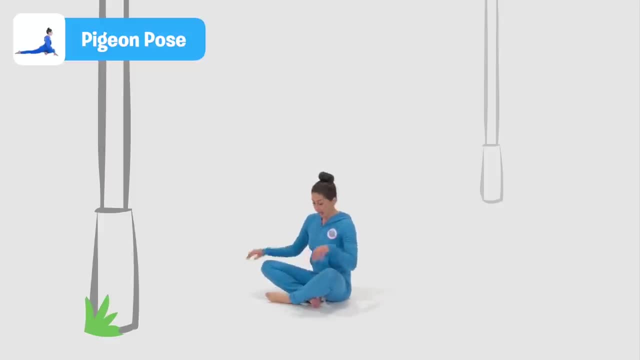 Sweeping that back leg all the way back forwards again and switching the cross on your legs, Bringing the other one in front. Yes, Now we're going to take that one forward. Take it round the side to the back and, as long as it can, be out the back. 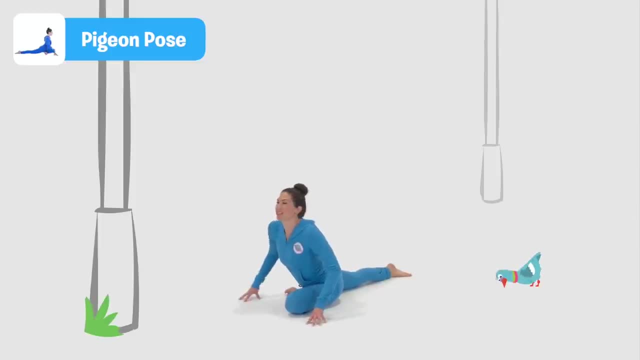 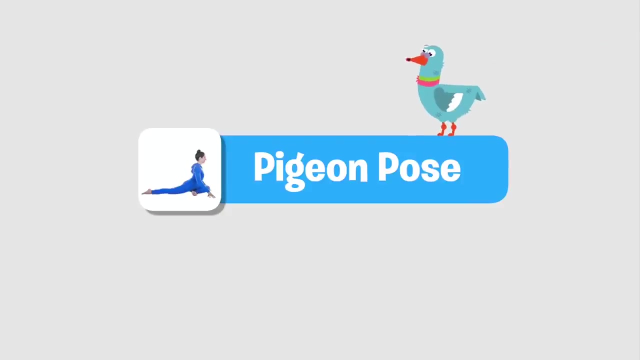 With this one at the diagonal line, again Up on our fingers, roll our shoulders back, Puffing up our chests going coo, coo, coo. Yes, exactly, I'm right with you on that. Pigeon pose, Tree pose. 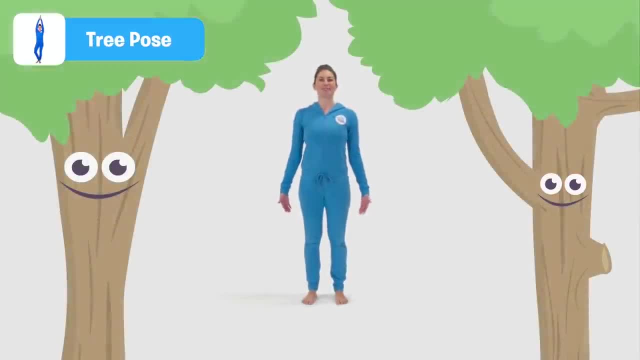 Standing nice and tall. We bring one leg forward, We bring one foot on top of the other, Using our heel, Our knee turns out to the side, We bring our hands together at our hearts And we grow our branches up nice and tall. 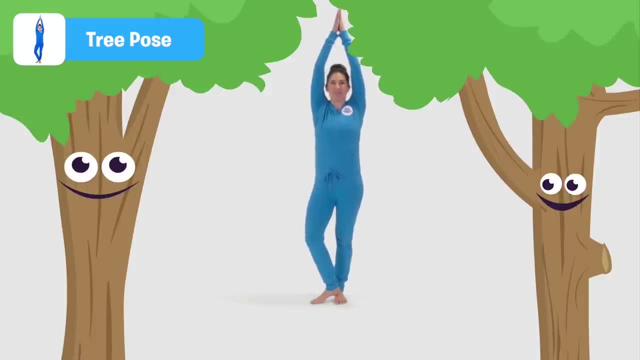 Stretching as high as we can. Wow. well done everyone. Now tree pose is really good for stretching our sides, Practising our balance And for strengthening our back and our legs. Well done, Now let's see if we can do it on the other side. 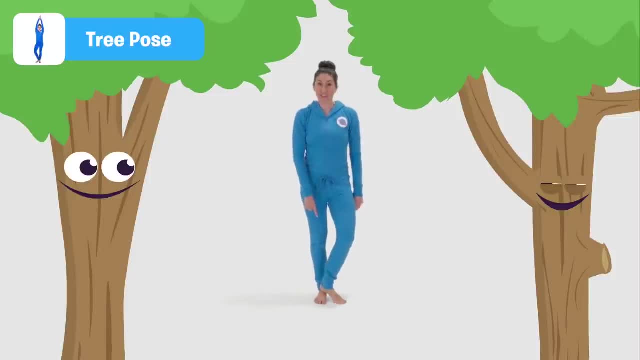 Lowering our arms all the way down. We switch our feet, so the other heel's on top. We bring our hands together. We grow our arms up. Our branch is nice and tall. Now I wonder how strong you trees are. I'm going to do the tree test.